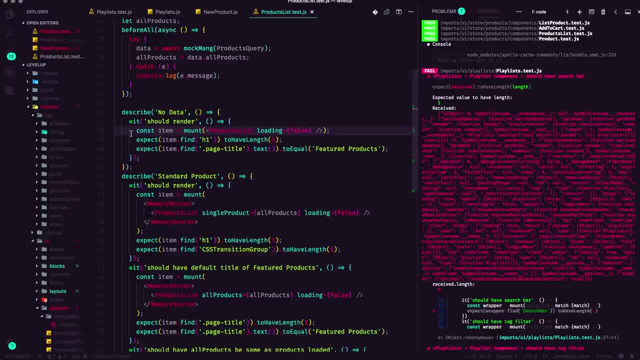 way, way more important in this sort of component based workflow, And that's testing how these things or units in our code interact with each other or how they integrate with each other. So instead of testing each individual component, we're going to be testing how they all work Now. 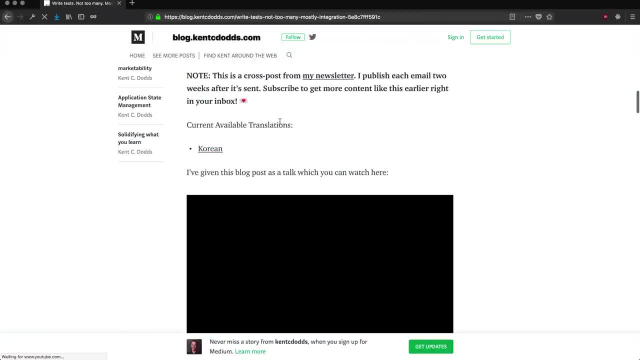 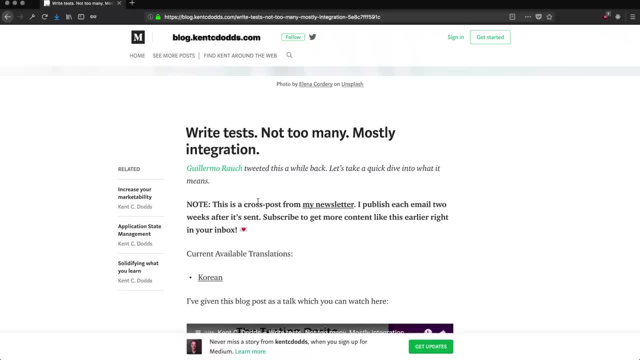 one of my favorite quotes is from Ken C Dobbs on his blog and he says: write tests not too many, mostly integration. And so that's a nice little quote to get this kicked off. Because what integration tests do in the sort of modern workflow is they make. 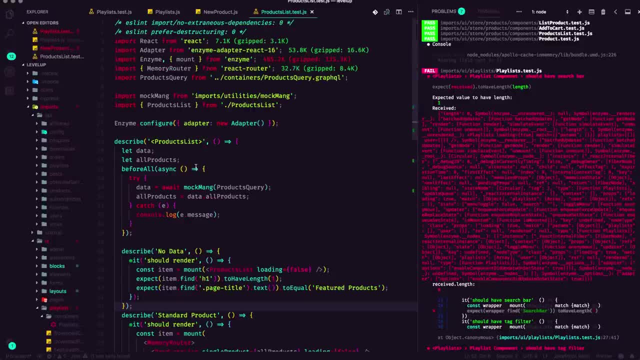 sure that things are working together. For instance, I'm using a library called enzyme to mount my react components. Now you could be using a shallow render which is only going to render that particular component. Let's take a look at this products list- component right. 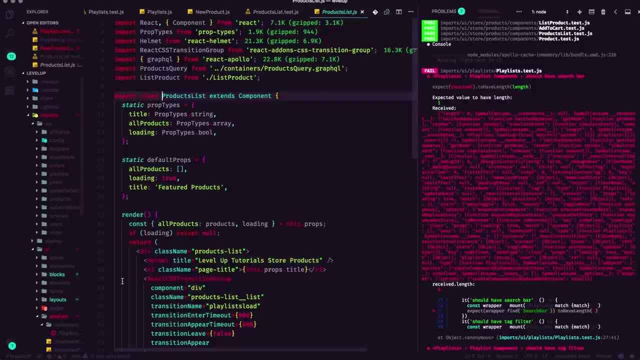 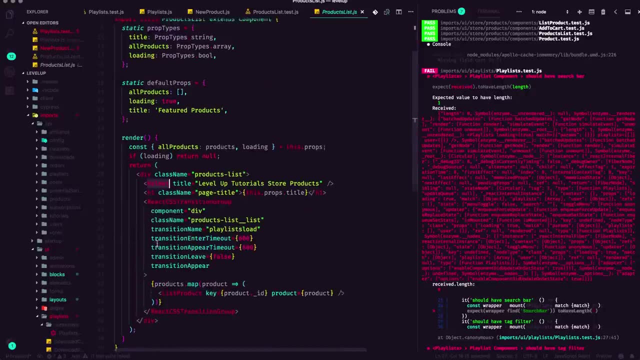 If we were to do a shallow, it's only going to render first thing deep, aka. it's not going to render into this react CSS transition group. Likewise, it's not going to render the helmet or it's not going to render any of our list products. it's just flat out not going to render them. it's just going to. 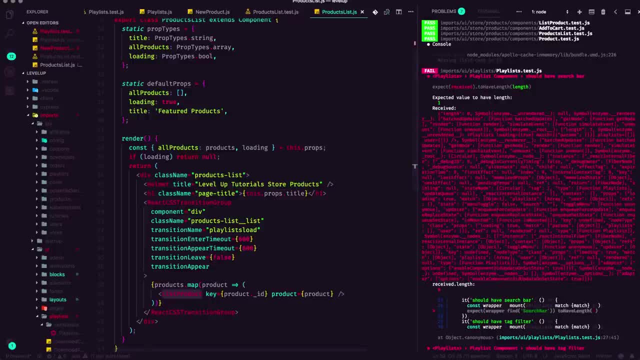 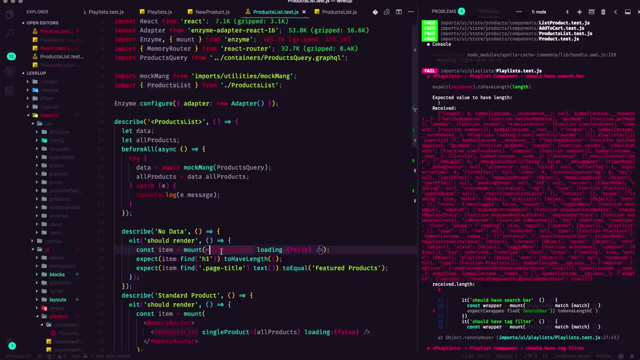 render this one. that would be a unit test. Now, with integration testings, we do something called a mount in enzyme, where we are mounting this component. Now, what mounting does, is it not only renders this component, but it also renders this component. So if we were to do a shallow 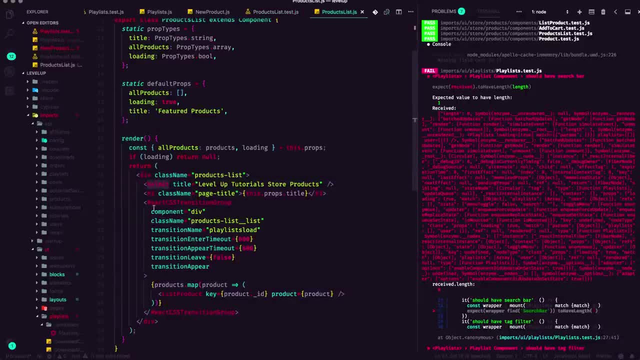 this component like this, but it also renders everything that's in helmet, everything that's in the react transition group, which is all of our list products, and it will render each of those out, as well as any sub components of that. If you think about it. it's really important to, because 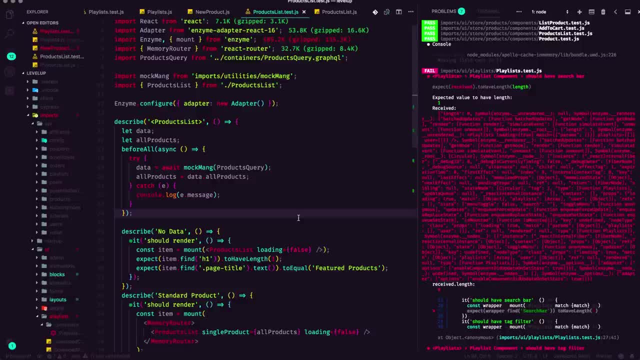 in your typical use, in your typical workflow. you very rarely are using your components in isolation. it's very rare that you would. in fact, it's impossible for me to essentially use this products list component without having the individual components. So if you were to do a 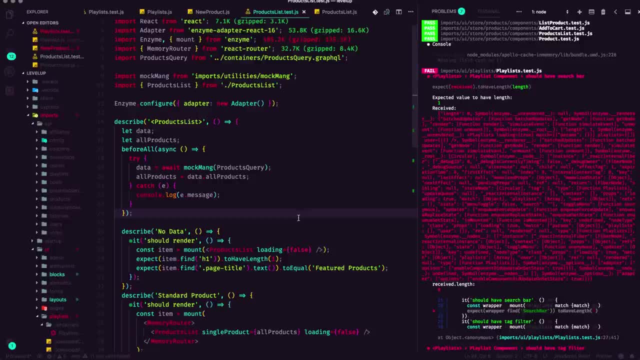 mount in enzyme. it's just flat out not going to render any of our list products. it's just going to have some sort of an impact on how the whole thing works right. So while I will write one unit test to make sure that the products list component is rendering as rendering the necessary things, 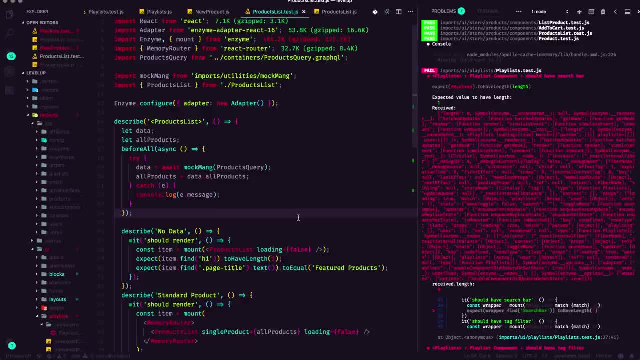 I'm going to be writing mostly integration tests so that I can see that this products list is in fact going to render correctly and that nothing, none of its sub components or child components, are going to get in the way of that rendering. And if you do that type of mounting for all of 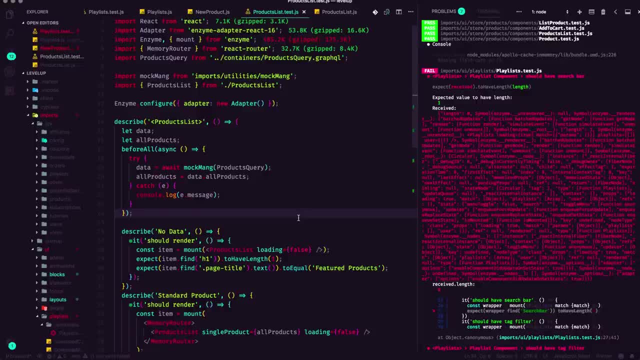 the components. you should know that they all integrate together in the actual real world use case, that you're using them in your application. So this is why integration testing is so important. So I mentioned again unit testing is testing an individual unit of your code where integration 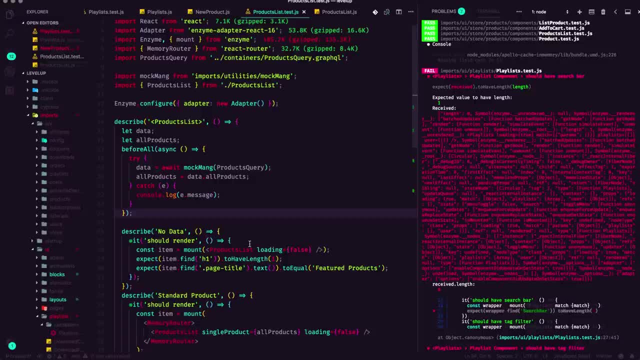 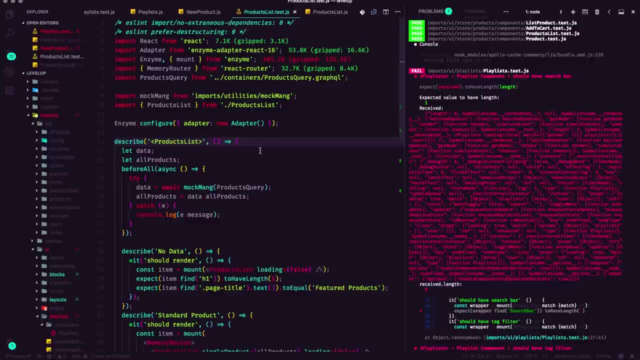 testing is testing how units of your code interact with each other, So that is integration testing. If you want to learn more about this kind of thing, let me know. in the comments I mentioned last time, I'm considering doing a course on testing. a lot of people were very, very excited about that, So I do intend on doing 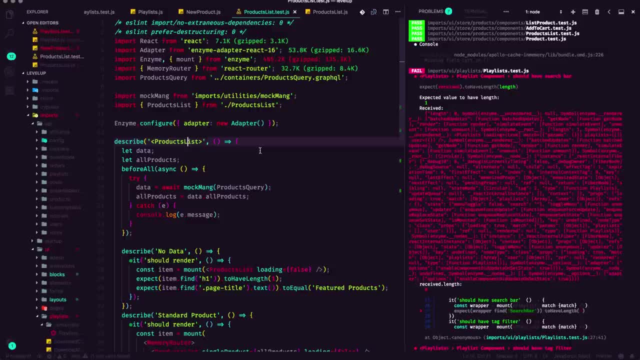 something involving testing. it most likely will be react based, most likely will have GraphQL components as well. Those could all be sort of separate, different components of the series. So let me know what you want to see out of a testing series. Let me know what you want to see out of the 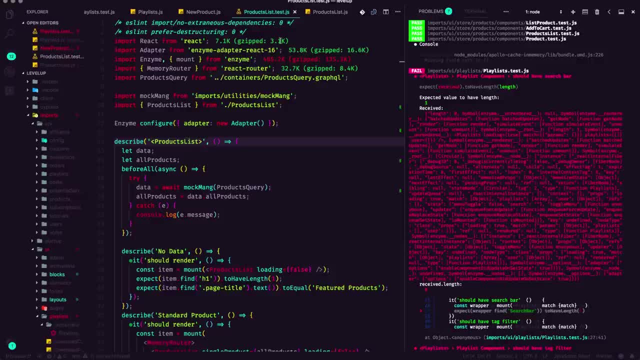 inevitable testing series here on Level Up Tutorials. So thank you so much for watching And let me know what else you want to see And what is Wednesday. I'm going to continue doing more what is Wednesday's on different types of testing as well, So look out for those next week and in the 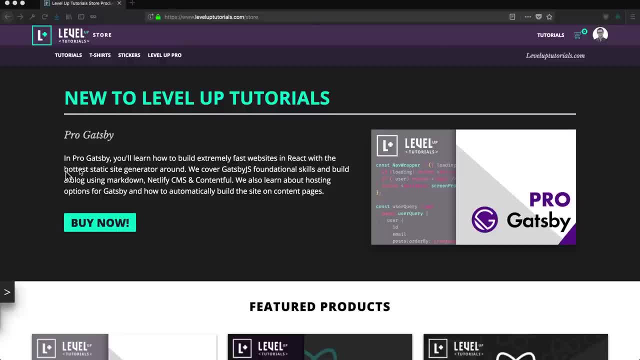 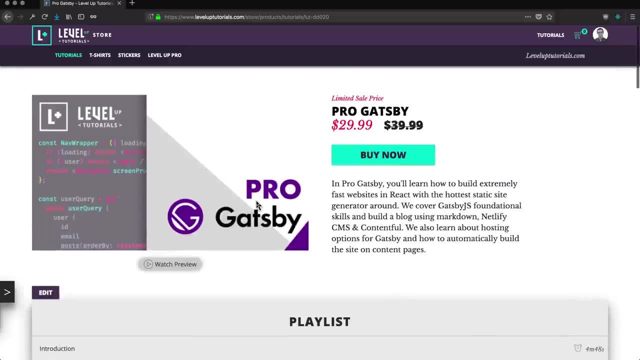 future. And one last thing: if you want to help support Level Up Tutorials, head on to leveluptutorialscom forward slash store and check out the latest pro series, which is pro Gatsby. Now you can buy this series individually and get access to all 25 videos on how to use Gatsby. the 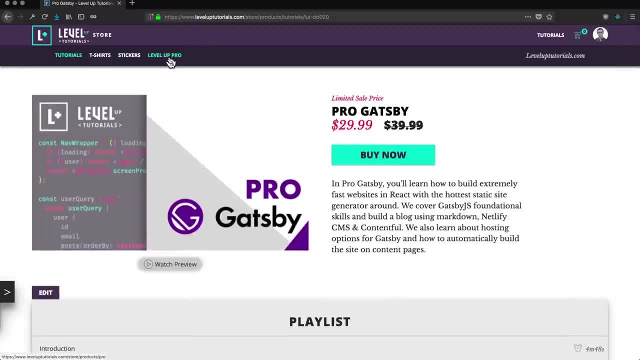 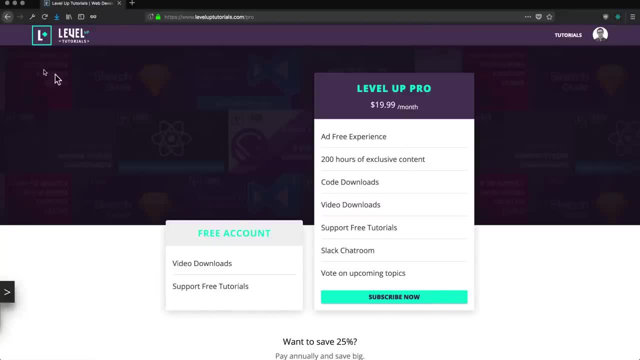 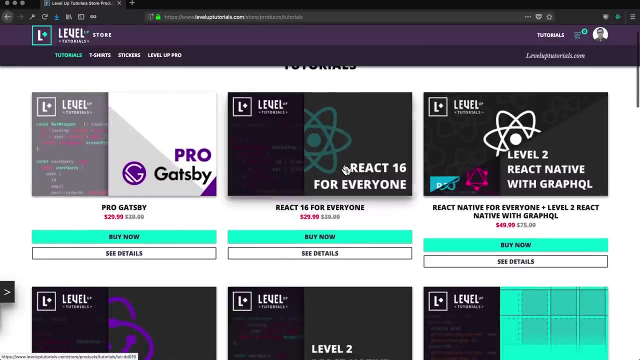 hot aesthetic side generator around. or you can become a level up pro by heading to level up tutorialscom forward slash pro, subscribing for 19 bucks a month and getting access to every single series that's available on the level up tutorial store, such as pro Gatsby, react, 16 for everyone. 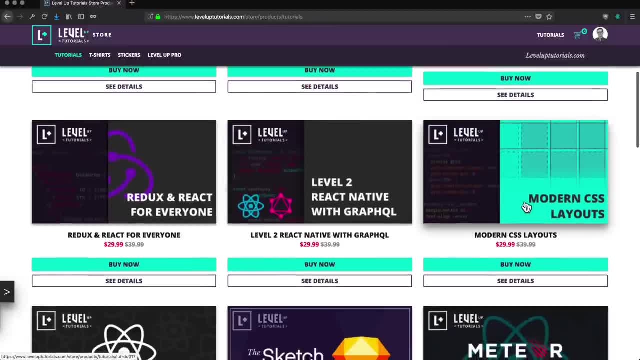 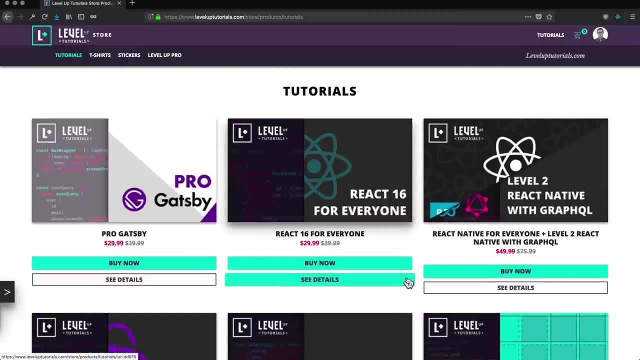 level to react, native react and redux modern CSS layouts- all this good, good stuff. So if you want to expand your mind with level up tutorials, head on over to leveluptutorialscom, forward slash store and check out everything that's available. Thanks so much for watching and I'll see you next week. the next one.